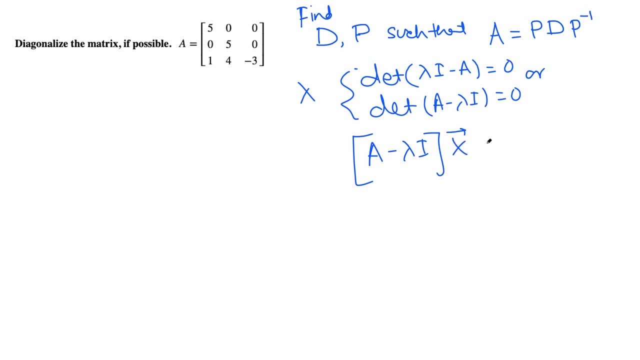 null space of A minus lambda I matrix or lambda I minus A same thing, and some vector, eigenvector- equals zero. so it's pretty much like Ax equals zero. so we are, we find the null space of this matrix matrix. So lower triangular means we can easily find the eigenvalues, okay. so 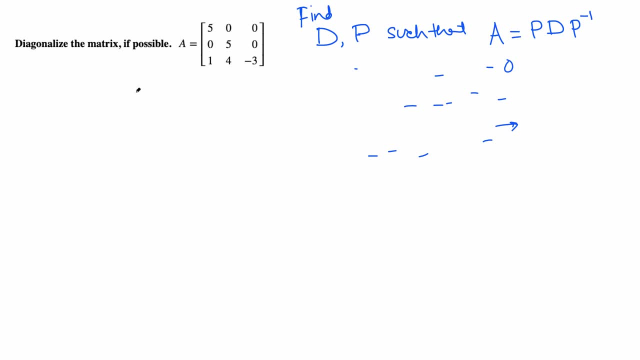 since a is lower, triangular eigenvalues are- let me write down lambda- 5, 5 and negative 3. so we can just say 5 and negative 3, so 5 with multiplicity of 2 and negative 3. so we got only two eigenvalues For this matrix to be. 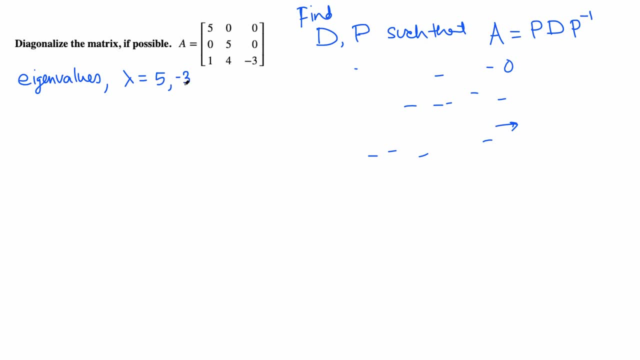 diagonalizable from these two. we, from these two eigenvalues we should be able to get, we need to get three linearly independent eigenvectors. so we have to have three eigenvectors If we find just one eigenvector from each of these two. 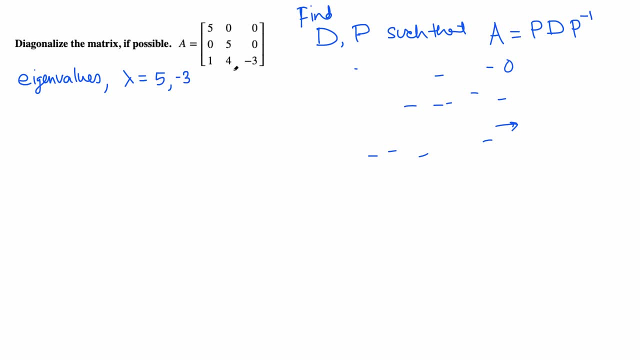 eigenvalues, then this matrix is not diagonalizable, So we must find three linearly independent eigenvectors. okay, So to find the eigenvectors, what we do is we just solve a minus lambda i: x equals 0, for lambda equals 5 and lambda equals negative 3.. So let me find this matrix. 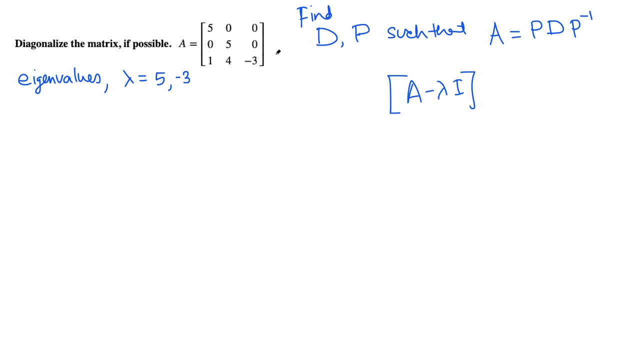 what is a minus lambda i? So a is the given matrix, i is the identity matrix, in this case three by three. so 1, 0, 0, 0, 1 0. so this is i and we multiply by lambda. so multiply each component, each element by lambda. so 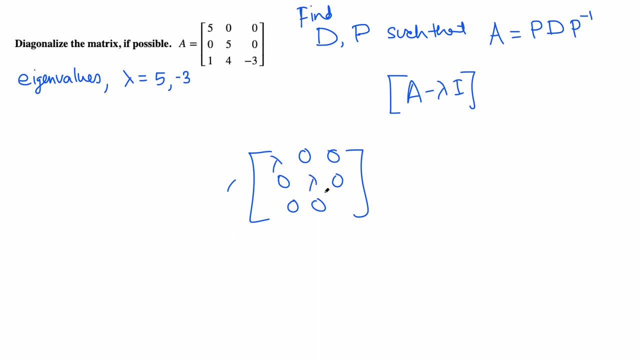 these three become just lambda, lambda, lambda. and we subtract this from a, so a is 5 0 0 0, 5 0, 1, 4 0.. negative 3, so a minus lambda i, which is I'm gonna write over here. we just: 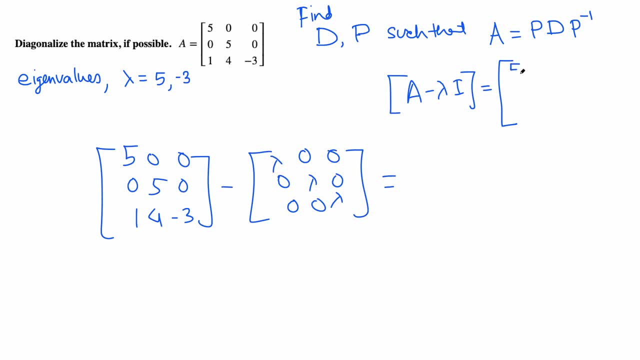 subtract the corresponding components: 5 minus lambda, 0 minus 0, just 0, 0. 5 minus lambda, 0, 1 minus 0, 1, 4 minus 0, 4, negative: 3 minus lambda. Okay, so we have this: a minus lambda i. now we take: lambda equals 5 and lambda. 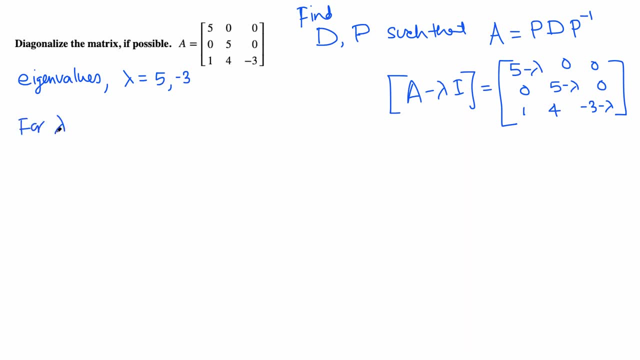 equals 3.. So first, for lambda equals 5, a minus lambda i. so we are trying to find the corresponding eigenvector. v or x, doesn't matter, equals 0. this implies- okay, I'm gonna write just the augmented matrix. so augmented matrix, so a minus lambda i is here, so we just replace. 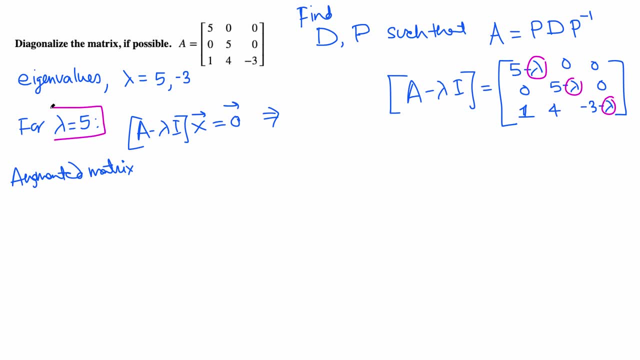 lambda by 5, okay, and that gives 5 minus 5, 0, 0, 5 minus 5, 0, 1, 4, negative 3 minus 5, negative 8, and that augmented means we don't need to write x, so 0, 0, 0. 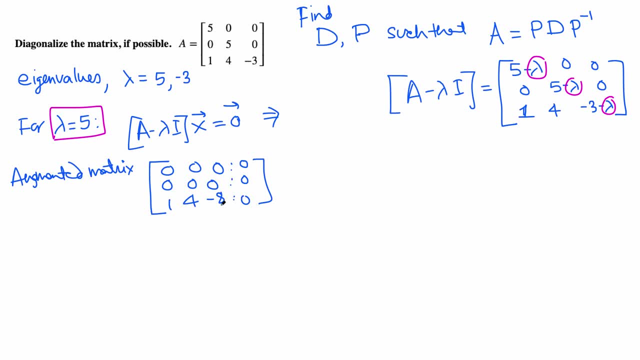 Now we do the row reduction and solve This. x got three components: x1, x2, x3.. Okay, so this one, 0, 0, 0, always on the bottom. so this one is same as- let me put this r3 in r1. so 1, 4, negative 8, 0 and doesn't matter- all zeros. 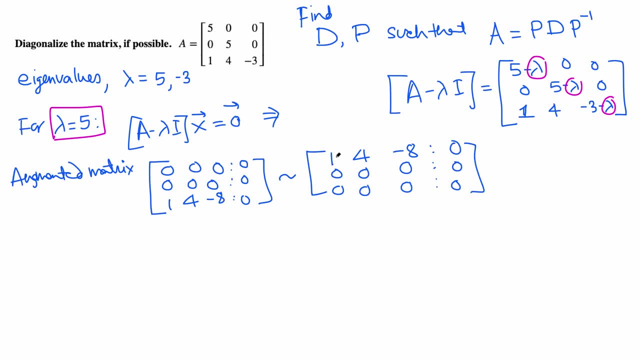 Now we got pivot here. this one is the pivot. there is no pivot here, no pivot. so this is x1, x2, x3. so no pivot here means x2 is a free variable, so is x3.. Now, solving this, we get x2 is just x2, x3 is just x3. from the first row we get 1x1, x2, x3.. 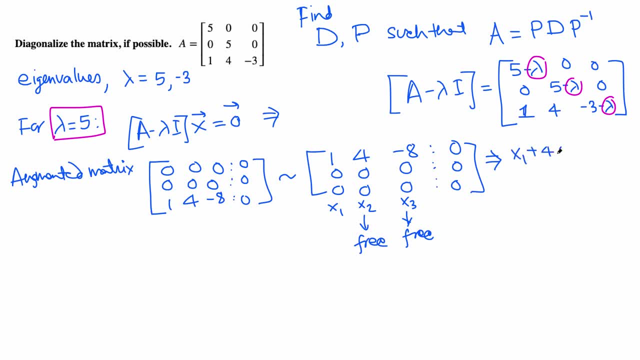 plus 4x2 minus 8x3 equals 0. Let's move this over and subtract and add. so our x1 is negative, 4x2 plus 8x3 and x2 and x3 are free. so this is. it So from this thus: 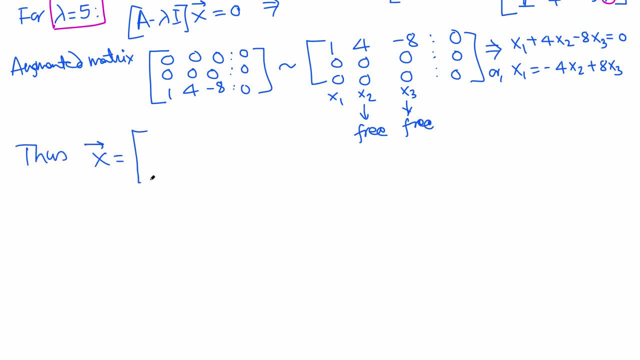 the corresponding eigenvector is just x1, x2, x3, which is x1, is found here negative 4x2 plus 8x3, x2 is just x2, because it's a free variable, and x3. If we look at closely here we got two types of arbitrary real numbers, because 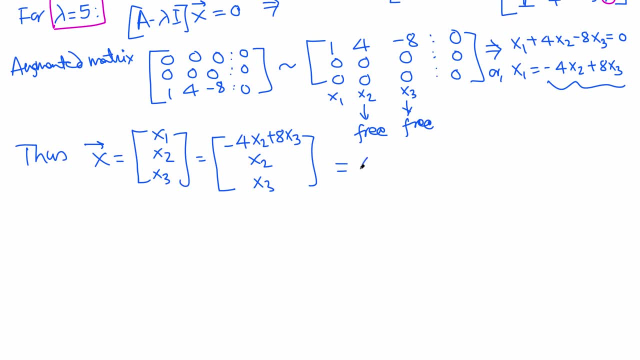 arbitrary real numbers x2 and x3, so I can factor x2 out and a vector plus x3 out and a vector. So x2 means here negative, 4x2, so negative 4 in the first component. x2 means 1, there is no x2, so just 0.. x3, oh 8x3, so 8 in the 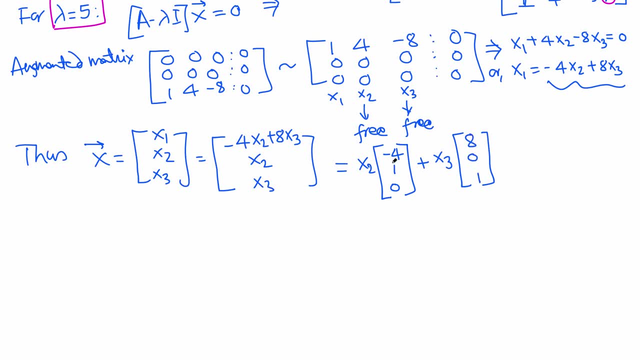 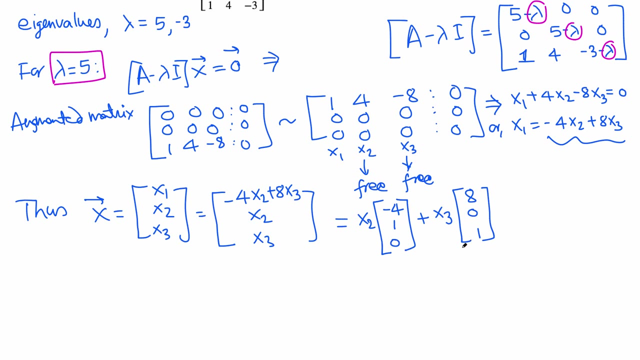 second component, non-zero. here is 1.. So the corresponding eigenvectors are here. So this is for the eigen space. we got two of them here, negative 410, 801, or these are the corresponding eigenvectors. So for lambda equals 5, we got two eigenvectors, and next we will find the 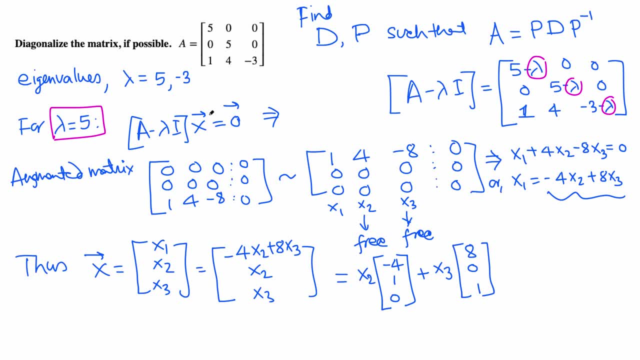 eigenvector corresponding to negative 3, and we are sure we get at least one. we always get at least one. Here we got 2 and we will get one more. that means we have two eigenvectors. that means a is diagonalizable and we'll find P and D. 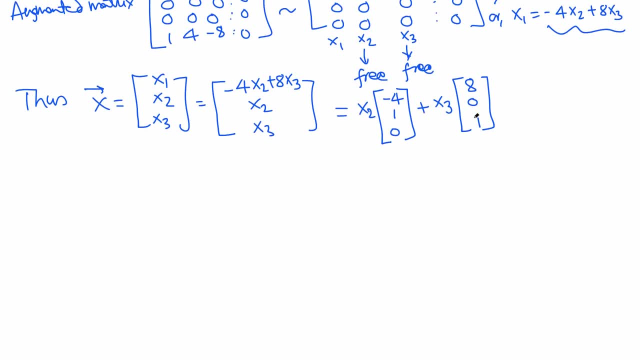 and B. okay, So thus. so, these are the eigenvalues. let me write in this way so we can just say: that's this one for lambda equals 5. the eigenvectors are: this one negative, 410, 801. okay, so I'm gonna write over here: 5 for 5. I got two of 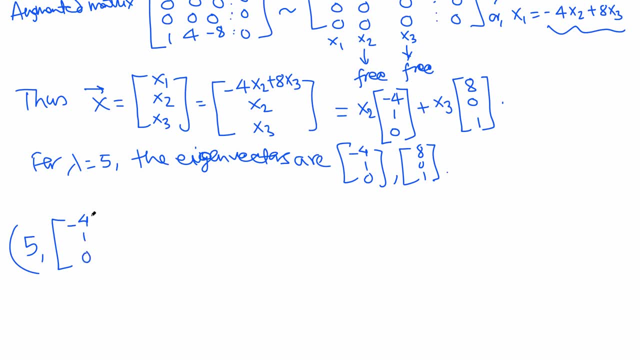 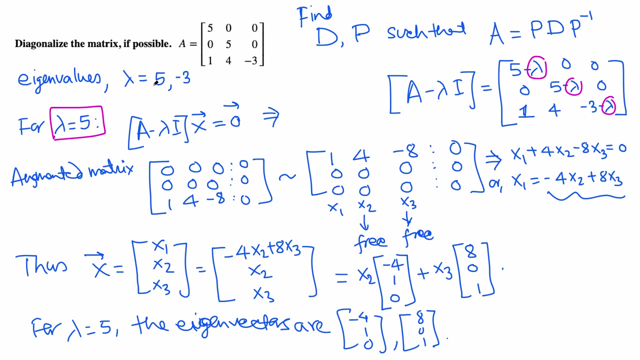 them negative: 410 and 801. okay, and now I'm gonna do the same work for 5. I got two. Now I'm gonna go over and just do the same work. for lambda equals negative 3. okay, So for lambda equals negative 3, we just plug in. 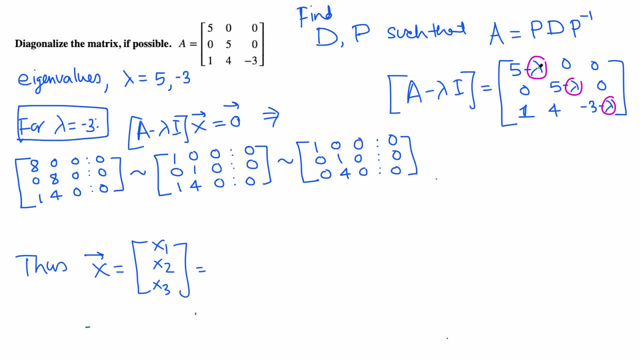 negative 3 for lambda here. so 5 minus negative 3 would be 8, 0, 0, 0, 8, 0, 1, 4, 0.. So we are here. so on the first row, I can multiply by 1, eighth, I get this second. 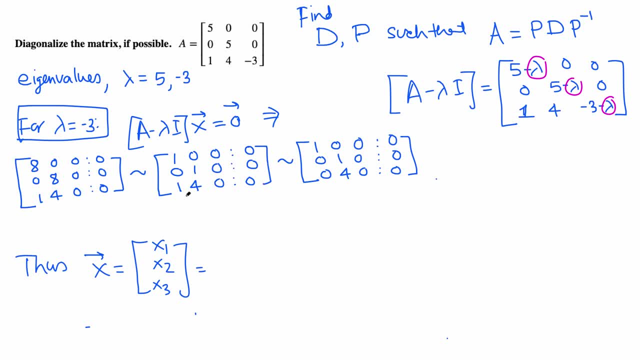 row. do the same thing, multiply by 1, eighth, I get this. and third row Now to change this into echelon form. so 1, 1. so I'm gonna move, I'm gonna work on r3 so that r3 plus negative 1 times r1, so 1 plus negative 1, 0 and we get this in the 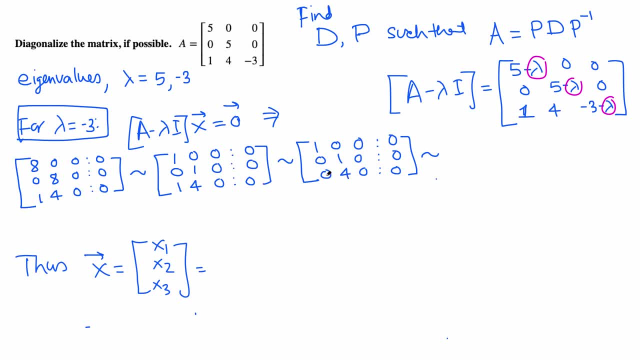 same way. now I can add r3 with negative 4 times r2 or multiply by negative 4 here and add with this. so it's gonna be 1, 0, 0, 0, 1, 0 and 0. so we are multiplying by negative 4, 4 plus negative 4 is 0 and everything is 0. so this is what we. 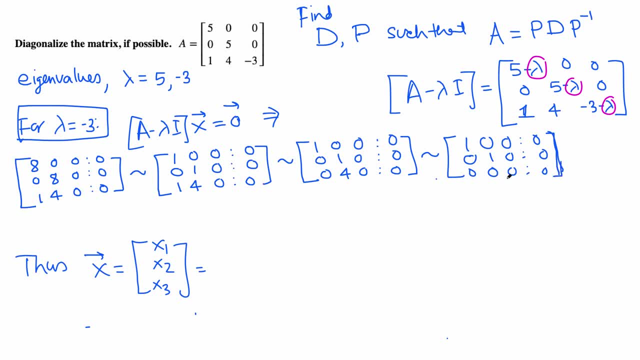 get. In fact, this is in reduced row echelon form. So here is a pivot 1,, here is another pivot, and this is x1,, x2, x3, and this is free variable because we don't have a pivot column. So this 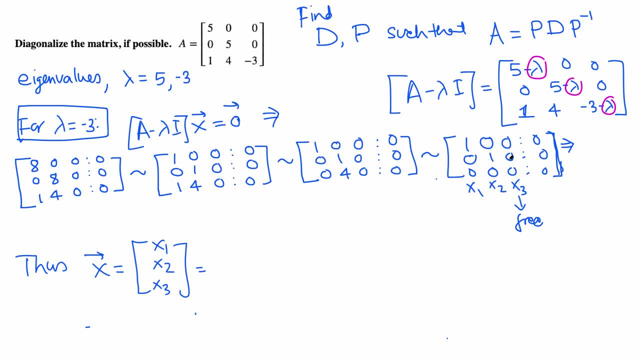 implies. in fact it's pretty simple here: x3 is free. look at, from the second row. from the second row we get 1 x2, x2 equals 0.. Okay, from the first row we get 1 x1 equals 0.. 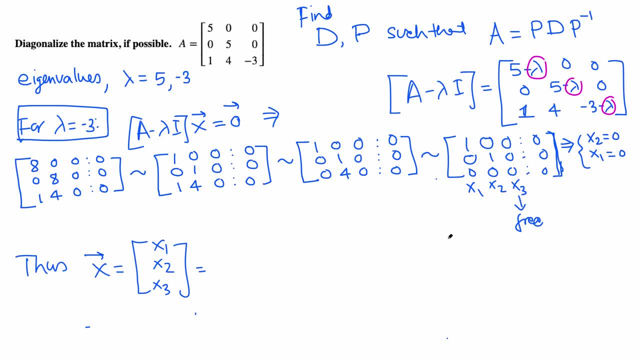 We get these two variables things and x3 is free. thus, like last time, we can we have: x is x1, x2, x3, which is in this case x1 is 0, x2 is also 0- look at here- and x3 is free, just x3. 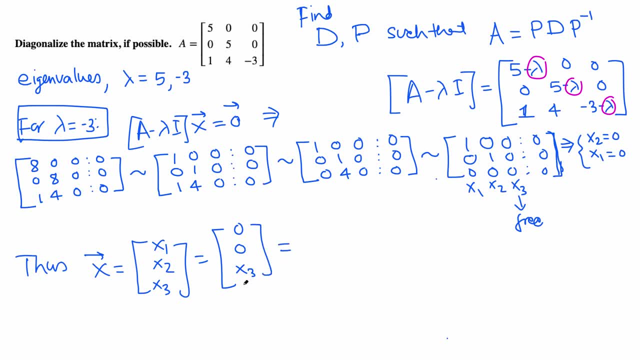 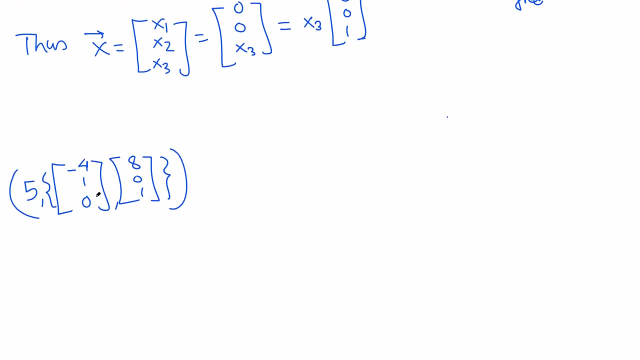 for now where x3 is arbitrary real number. so we can just factor x3 out, we get 0 0- 1 as the basis for the eigen space or corresponding eigen vector. 0 0- 1 is the corresponding eigenvector for the eigenvalue. lambda equals negative 3.. So last time I left here for 5, we got 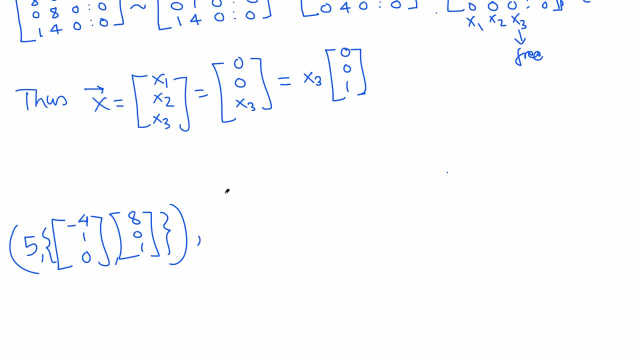 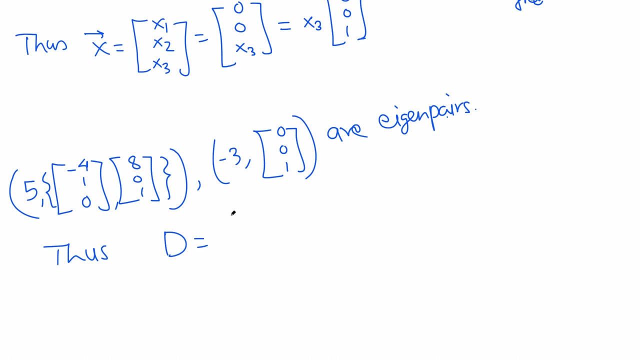 two eigenvalues and I just found for negative 3. I got 1, 0, 0, 1 as eigenvector, value, eigenvector: okay, these are eigen pairs. we can say in this way: then plus d, the diagonal matrix is just the eigenvalues. so 5, we got 2, so we need to write 5 twice. 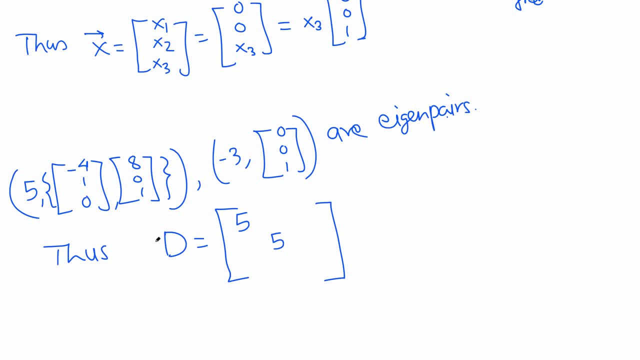 because 5 got 2 eigenvalue eigenvectors and negative 3.. Or you can write negative 3 first, doesn't matter, and all others zero, because it's a diagonal matrix. and when we have a diagonal matrix we can multiply this easily. later you can exponentiate when you are doing. 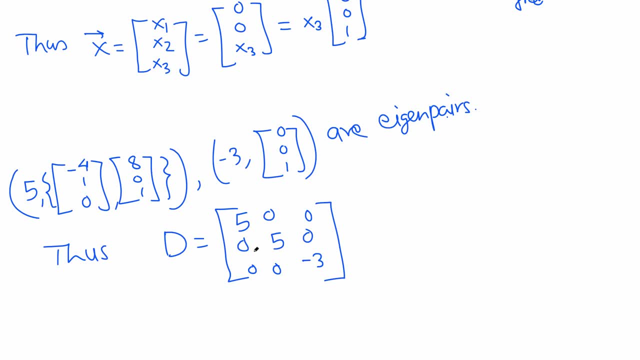 differential equations. so this is really easy to handle. and the p, the p matrix will be. look at this: 5, this 5. now we can write one of these two eigenvectors. so 5 means let's write one of them, negative. 4. 1- 0 is a column and for 5 another.